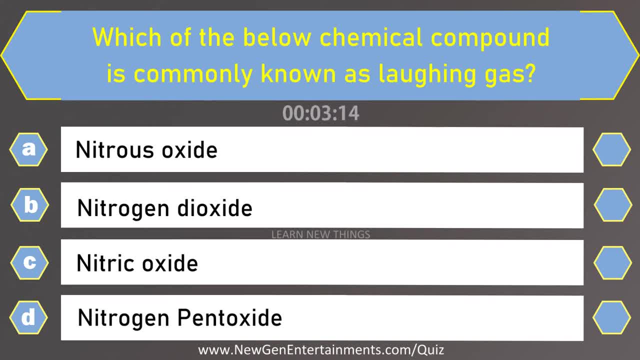 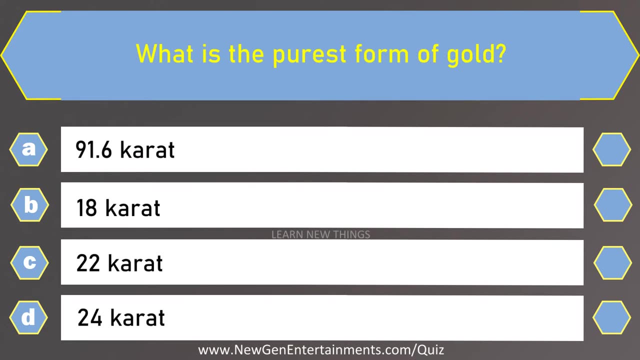 B- Nitrogen Dioxide, C- Nitric Oxide and D- Nitrogen Pentoxide. Answer is Option A- Nitrous Oxide. What is the purest form of Gold? Options are A- 91.6 Carat, B- 18 Carat, C- 22 Carat and D- 24 Carat. 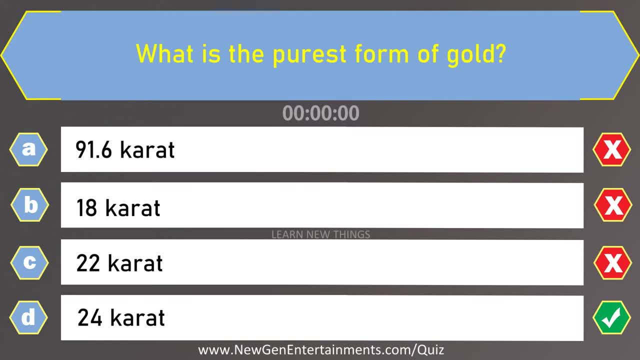 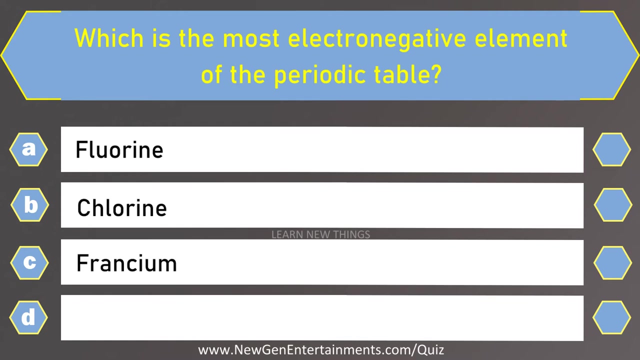 Answer is Option D, 24 Carat. Who discovered neutrons? Options are A- Ernest Rutherford, B- James Chadwick, C- JJ Thompson and D- Eugen Goldstein. Answer is Option B, James Chadwick, Which is the most electronegative element of the periodic table. 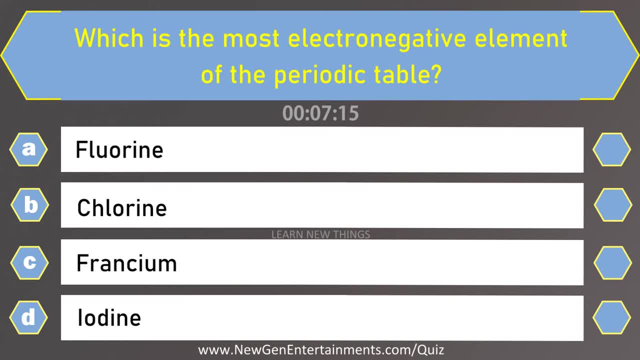 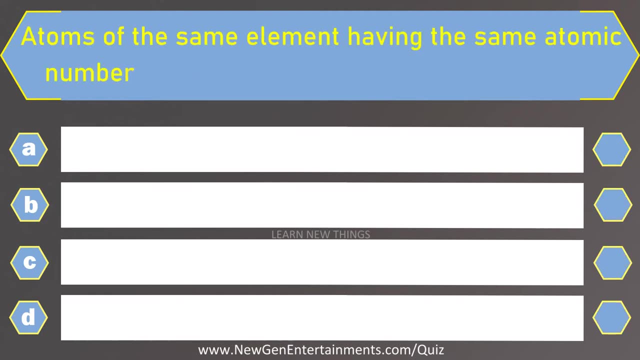 Options are: a- Fluorine, b- Chlorine c, Fransium, d- Iodine. Answer is Option a: Fluorine. Atoms of the same element having the same atomic number but different mass numbers are called. options are: a- Isotons, b- Isomerism. 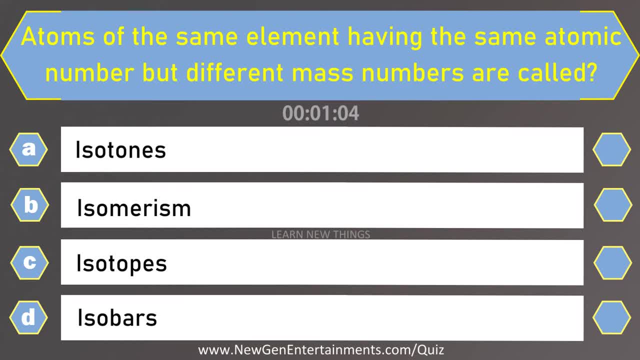 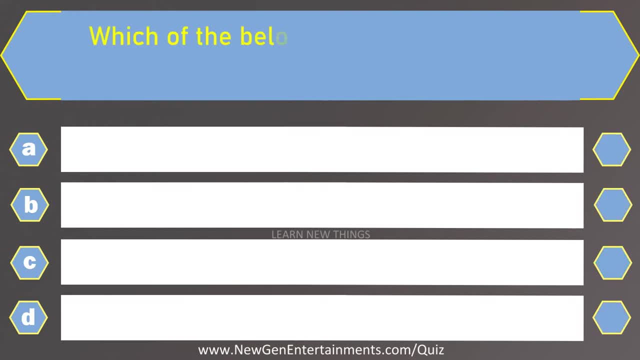 c- Isotops, d- Isobars. Answer is Option c- Isotops. Which of the below elements is used for the making solar cells? Options are: a- Sodium b, Magnesium c, Calcium d, Silicon. Answer is Option d, Silicon. 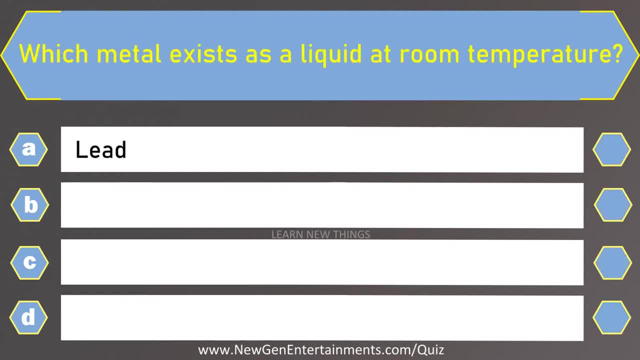 Which metal exists as a Liquid at room temperature? Options are a- Lead, b- Mercury, c- Gold, d- Zinc. Answer is Option b- Mercury. What is the chemical name of baking soda? Options are a- Sodium bicarbonate, b- Sodium chloride. 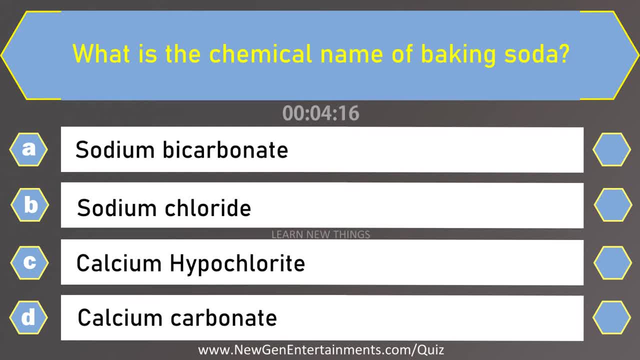 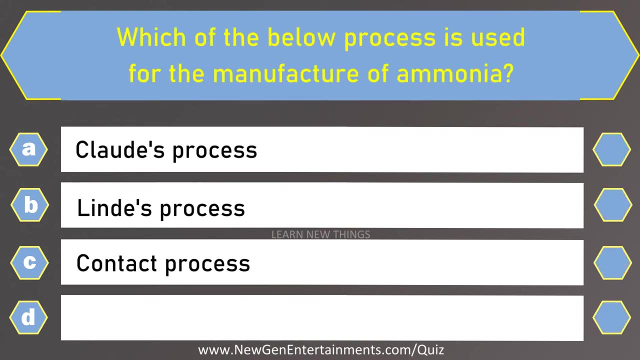 c- Calcium hypochlorite, d- Calcium carbonate. Answer is Option a, Sodium bicarbonate. Which of the below process is used for the manufacture of ammonia? Options are: a- Clouds process. b- Lindase process. c- Contact process. d- Haber process. 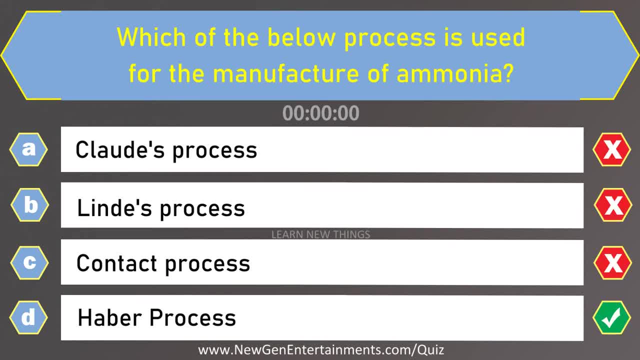 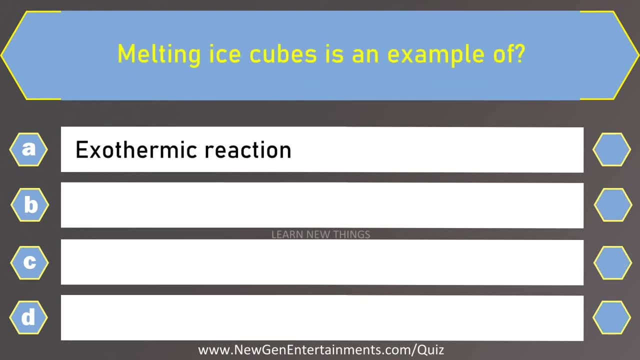 Answer is Option d- Haber process. Option a- Clouds process. b- Lindase process. c- Contact process. d- Haber process. Answer is Option d- Haber process. Melting ice cubes. Melting ice cubes is an example of Options. are a Exothermic reaction. 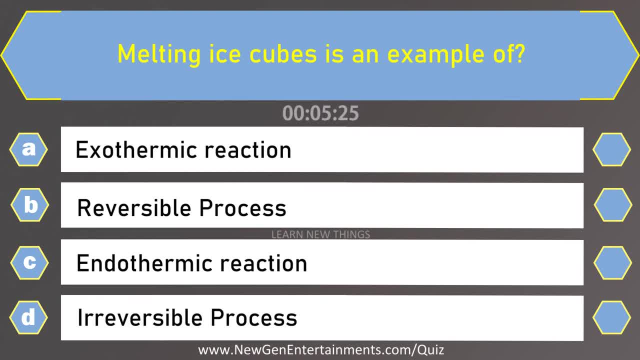 b- Reversible. step c- Endothermic. Jackson d- Irreversible process. Answer is Option c, Endothermic reaction. How many atoms per unit cell are there in a phase-cended cubic biomass? In this example, we will get an answer. 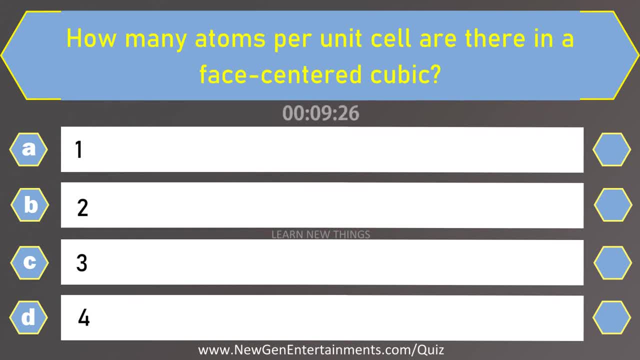 Harlem indexing the epsilon values in climate milk in 1 unit cellifer standard cubic Options are A: 1, B, 2, C, 3 and D, 4.. Answer is Option D 4. Hydrogen peroxide is a powerful dash agent. 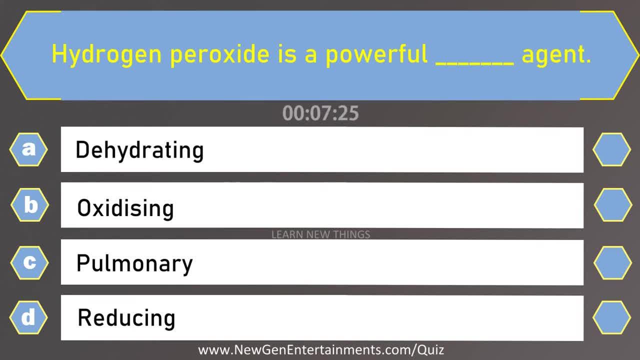 Options are: A- Dehydrating, B- Oxidizing, C- Pulmonary, D- Reducing. Answer is Option B- Oxidizing. Who is known as the father of nuclear physics? Options are: A- Ernest Rutherford B James. 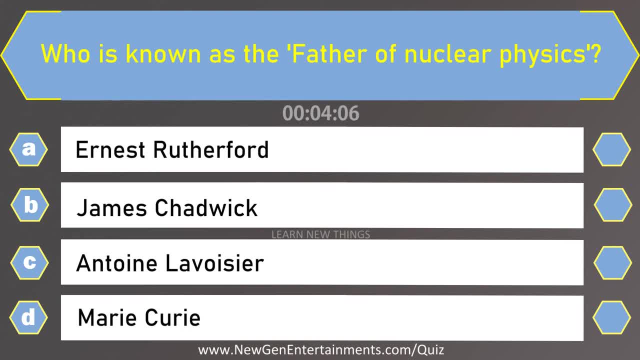 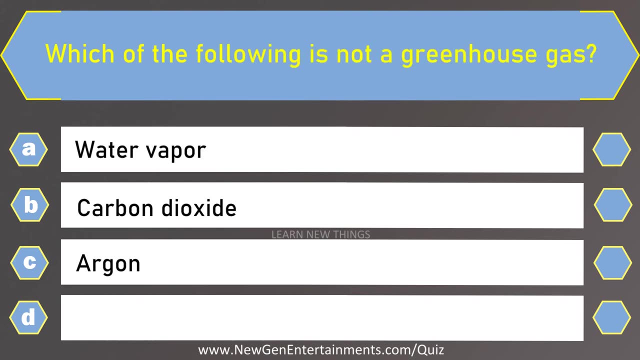 Chadwick C. Antoine Lavoisier, D- Mary Query. Answer is Option A, Ernest Rutherford. Which of the following is not a greenhouse gas? Options are: A- Water vapor, B- Carbon dioxide, C- Orgon, D- Osone. 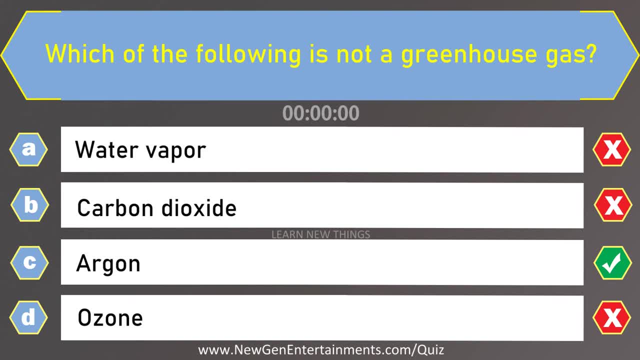 Answer is Option C, Orgon, Which inner elemento in our system contains carbon. Why water? P 혼자 Ogronda bathtub M An Either buy drink or is tried wrong. gas is used in beacon lights. Options are A- Argon, B Radon, C Krypton and D Neon. 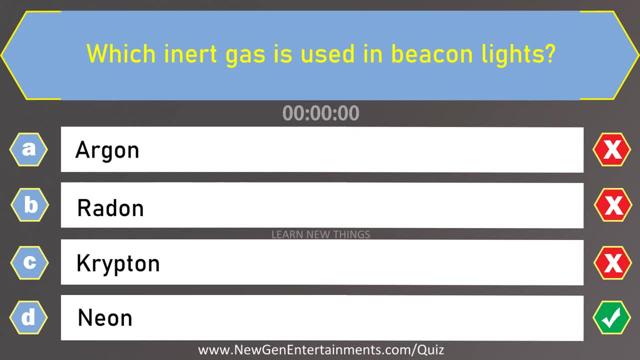 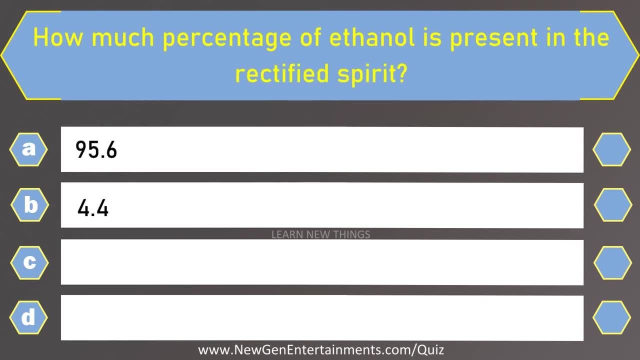 Answer is Option D- Neon. How much percentage of ethanol is present in the rectified spirit? Options are A 95.6, B 4.4, C 100 and D 90.7.. Answer is Option A 95.6.. 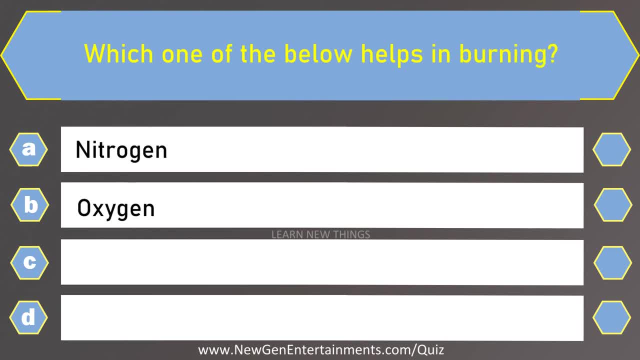 Which one of the below helps in burning? Options are A- Nitrogen, B- Oxygen, C- Carbon Dioxide and D- Carbon Monoxide. Answer is Option B- Oxygen, Which gas is used to accelerate the ripening process of fruits? Options are A- Methane. 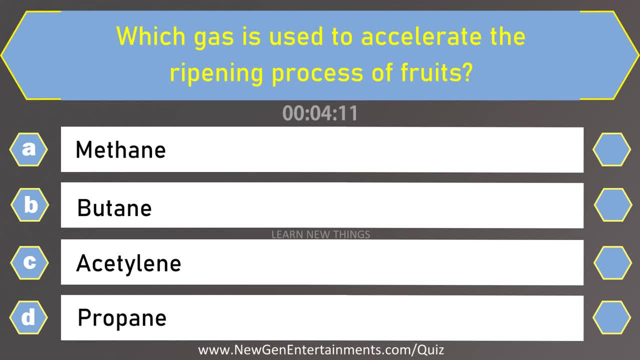 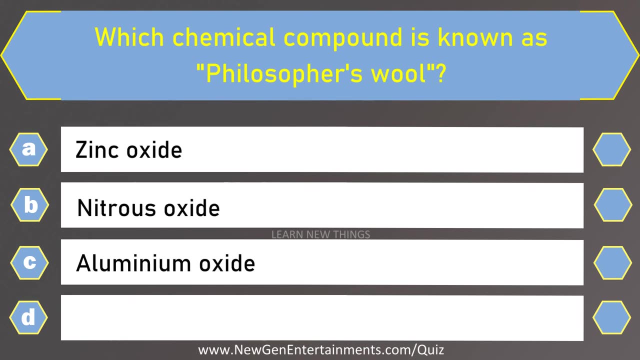 B- Butane, C- Acetylene, D- Propane. Answer is Option C- Acetylene. Which chemical compound is known as Philosopher's Wool? Answer is Option D- Oxygen. Which chemical compound is known as Philosopher's Wool? 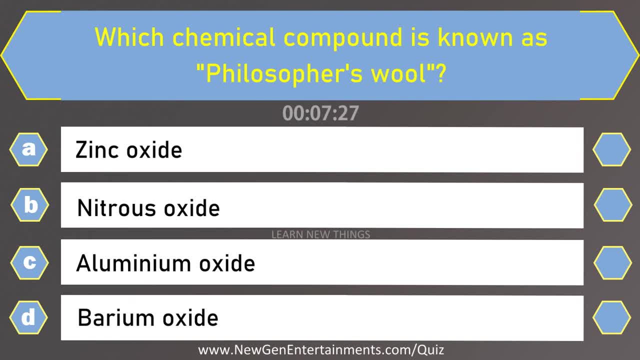 Answer is Option C- Oxygen, Which chemical compound is known as Philosopher's Wool? Options are A- Zinc Oxide, B- Nitrous Oxide, C- Aluminium Oxide and D- Barium Oxide. Answer is Option A- Zinc Oxide. 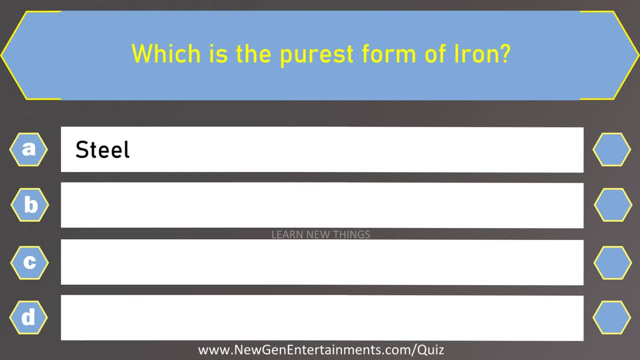 Which is the purest form of iron? Options are: A- Steel, B- Cast Iron, C- Brote Iron, D- Pig Iron. Answer is Option C- Brote Iron. Which of the below is an ore of aluminium? Options are: A- Thymotite, B- Coal, C Pyrate, D- Bauxite. 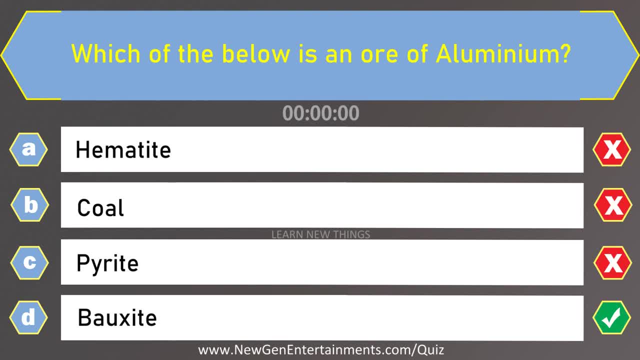 Answer is Option D, Bauxite. Answer is Option D, Bauxite. Which molecule solids toxic? Which molecule solids toxic? Answer is Option C- Homazdecapeab. Answer is Option D: Hirmidoidog GREGOR. Answer is Option C, Hirmidoidog Cuz eight days of Laurence dillancus from wisat. It claims by the administration that 11ZYG orIVEんな camy, affiliated to a позволment factor of CONDITbut of oxy- immature orientated yourself.